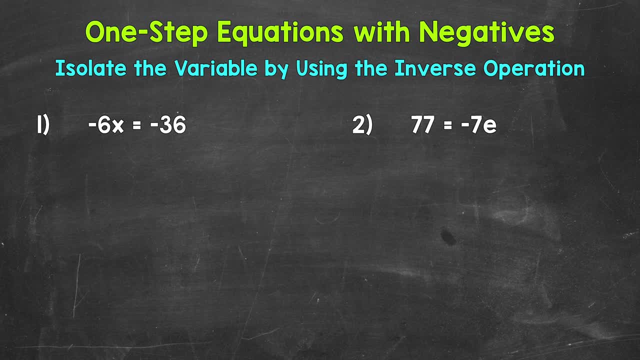 Just remember: whatever is done to one side of the equation, it must be done to the other in order to keep everything balanced and equal. Let's jump into number one, where we have negative 6x equals negative 36.. Now we have a number next to a variable. That means we are multiplying. 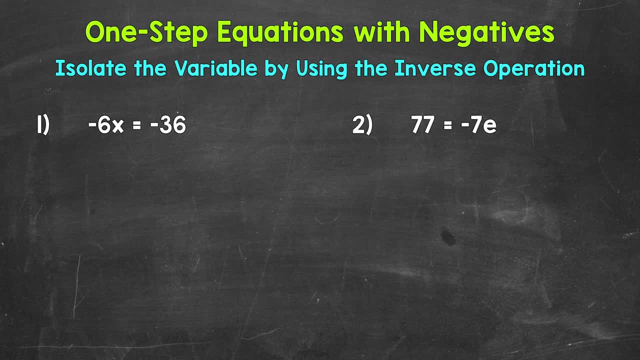 This is negative. 6 times x equals negative 36.. So whenever you see a number next to a variable, that is representing multiplication, So something to do with multiplication. Now we need to isolate that variable of x. We need to figure out what x equals. 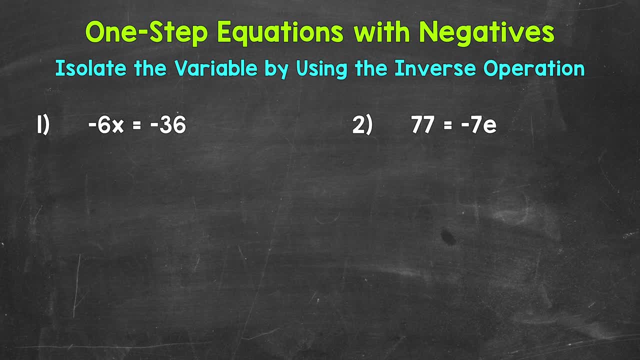 Since x is being multiplied by negative 6, we need to undo that multiplication by using the inverse operation. So the opposite operation, The opposite of multiplication, is division. So let's divide the left side of the equation by negative 6.. 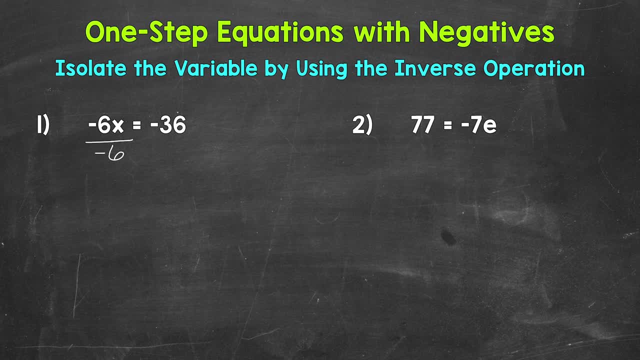 Whatever we do to one side of the equation, we must do to the other in order to keep it balanced and equal. So let's divide the right side by negative 6 as well. Now let's take a look at the left side of the equation. 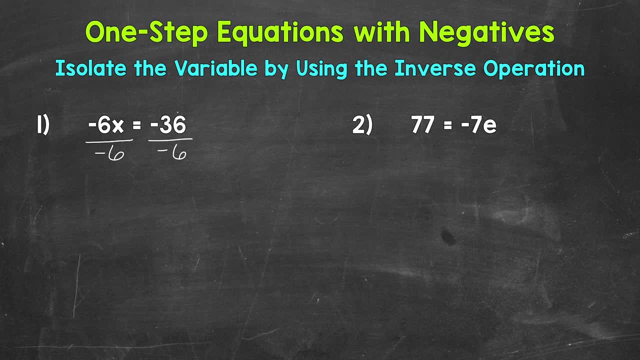 We are multiplying by negative 6 and dividing by negative 6.. So these negative 6's cancel out. They equal a positive 1, because we have negative 6 divided by negative 6.. A negative divided by a negative equals a positive, so we end up with a positive 1.. 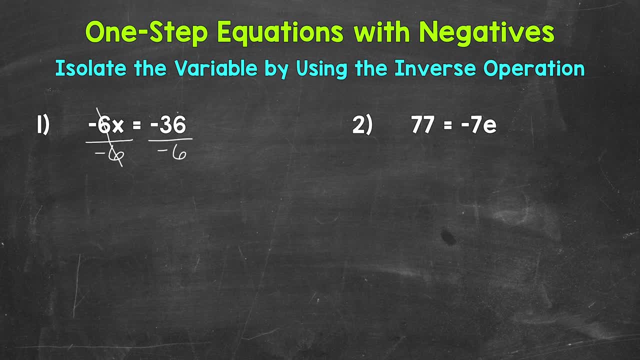 This gives us 1x, which is just x. So x is now isolated. It's by itself x equals. and then, on the right side of the equation, negative 36 divided by negative 6 equals a positive 6.. 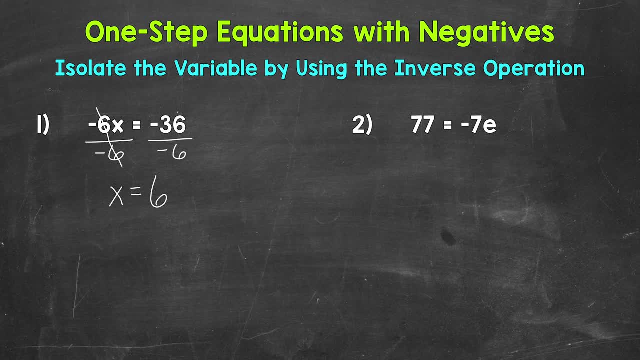 Because, again, a negative divided by a negative equals a positive. So this is our solution: x equals 6.. Now we can always check a solution by plugging it into the original equation. So let's plug 6 in for x and see if this works. 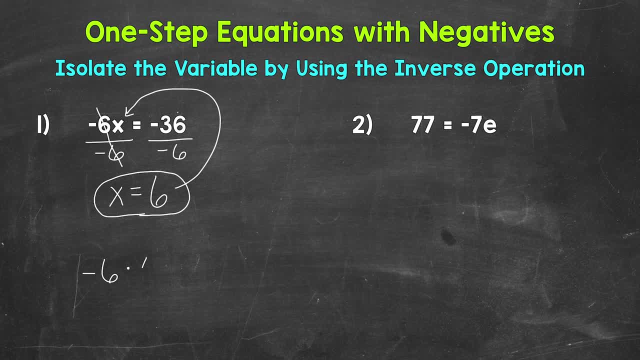 So we have: negative 6 times a positive. 6 equals negative 36. A negative times a positive equals a negative. So negative 6 times a positive 6. does equal negative 36. We have the correct solution. 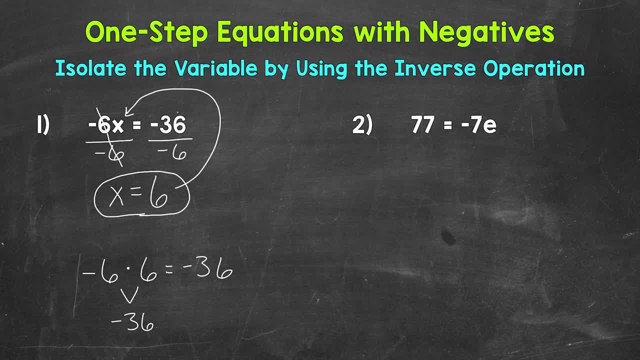 x equals 6.. Let's move on to number 2, where we have 77 equals negative 7e. So we need to isolate that variable of e. e is being multiplied by negative 7. We need to undo that multiplication by using the inverse operation. 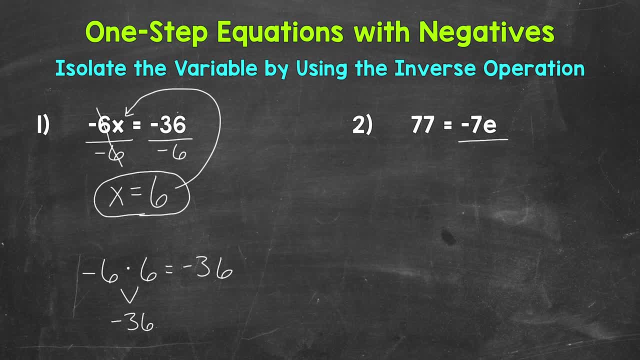 The inverse of multiplication is division. So let's divide The right side by negative 7.. Whatever we do to one side of the equation, we must do to the other. So let's divide the left side by negative 7 as well. 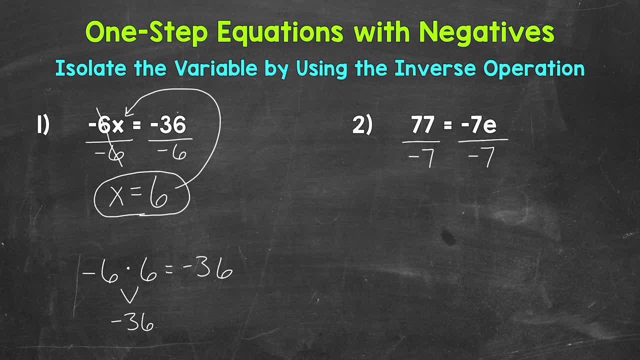 Now taking a look at the right side of the equation. we are multiplying by negative 7 and dividing by negative 7.. So these negative 7s cancel out. They equal 1. We have negative 7 divided by negative 7.. 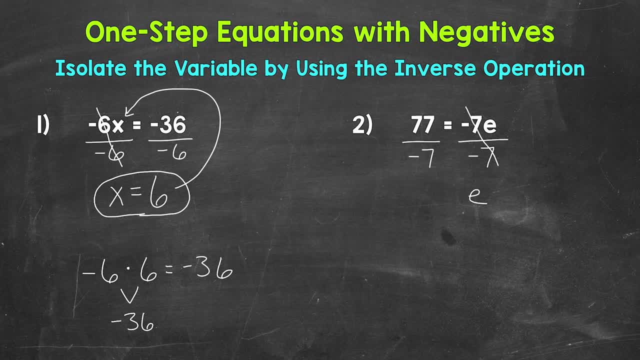 That gives us 1e, Which is just e. Our variable is now isolated. It's by itself e equals. And then on the left side of the equation, we have 77 divided by negative 7. So a positive divided by a negative. 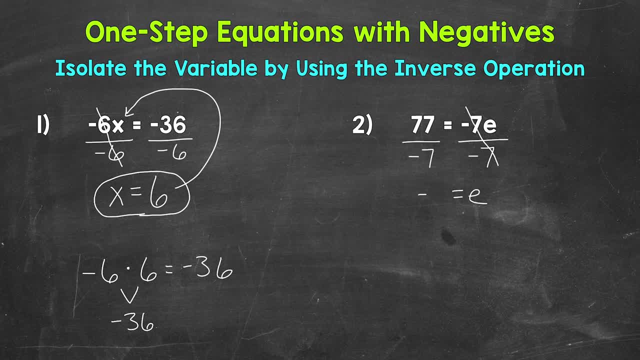 That's going to equal a negative, So we get negative 11.. e equals negative 11.. And we can rewrite this with the variable coming first. So e equals 11.. Negative 11.. Let's check that solution by plugging negative 11 in for e. 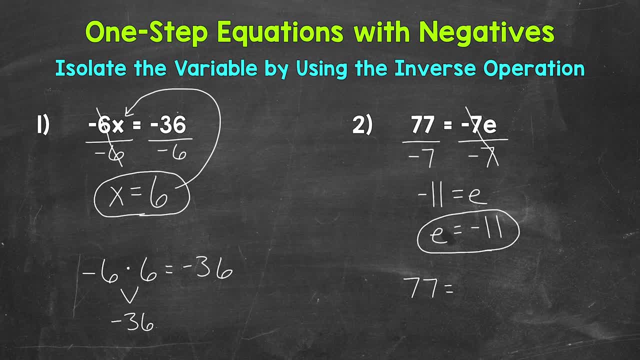 So we have 77 equals negative, 7 times negative, 11. We have a negative times a negative Negative, 7 times negative, 11. A negative times a negative equals a positive, So negative, 7 times negative, 11. Does equals 77.. 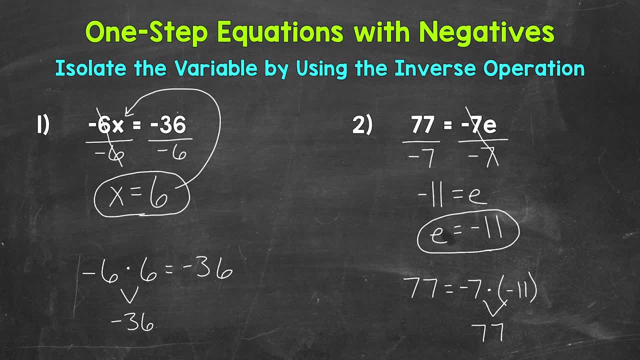 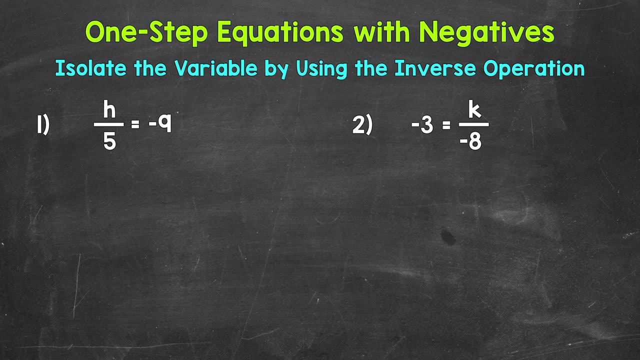 A positive 77. We have the correct solution: e equals negative 11.. There's how we solve one step multiplication equations with negatives. Let's move onto division. Here are our examples of one step division equations with negatives. Let's jump into number 1, where we have 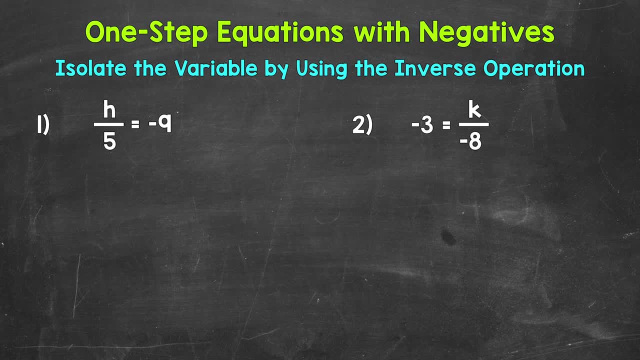 h divided by 5. equals negative 9.. Now we need to isolate that variable of h. We need to figure out what h equals. Since h is being divided by 5, we need to undo that division by using the inverse operation. 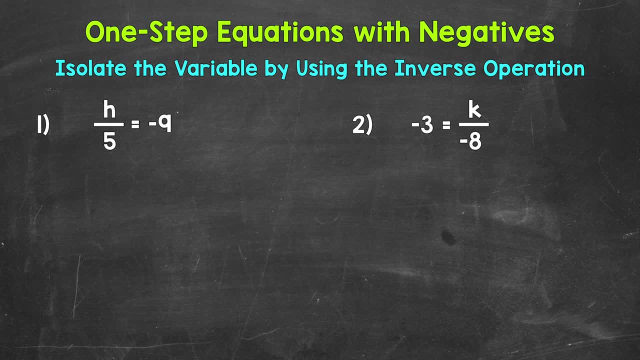 So the opposite operation, the opposite of division, is multiplication. So let's multiply the left side of the equation by 5.. Now, whatever we do to one side of the equation, we must do to the other in order to keep it balanced and equal. Let's multiply the right side. 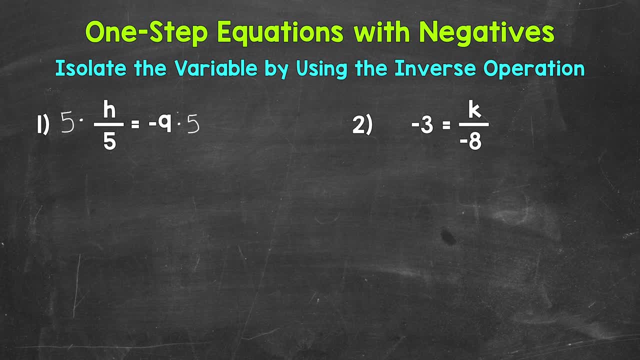 of the equation by 5 as well. Now let's take a look at the left side of the equation. We are dividing by 5 and multiplying by 5.. So these 5s cancel out. They equal 1.. Now let's take a look at the left side of the equation. We are dividing by 5 and multiplying by 5.. 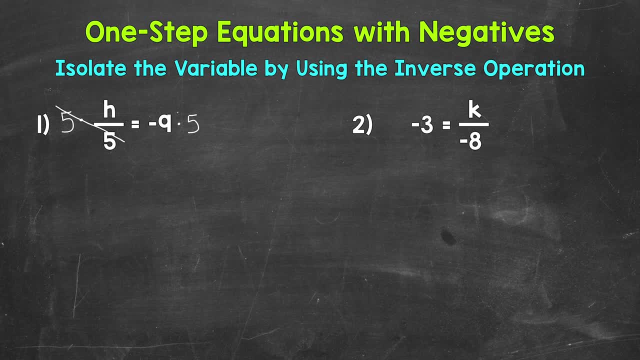 1, because when we multiply h divided by 5 by 5, we end up with 5h over 5.. We have 5 divided by 5, which gives us that 1, and then we have the h. We end up with 1h, which is just h, Our variable. 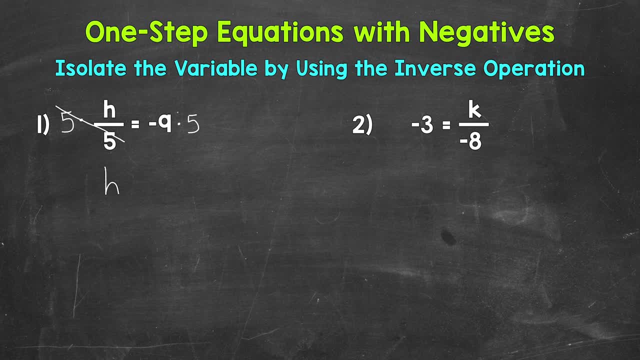 is now isolated. h is by itself, so h equals. and then on the right side of the equation, we have negative 9 times 5.. We have a negative times a positive, which equals a negative. so this equals negative 45. h equals negative 45. That's our solution. Now we can always check a solution. 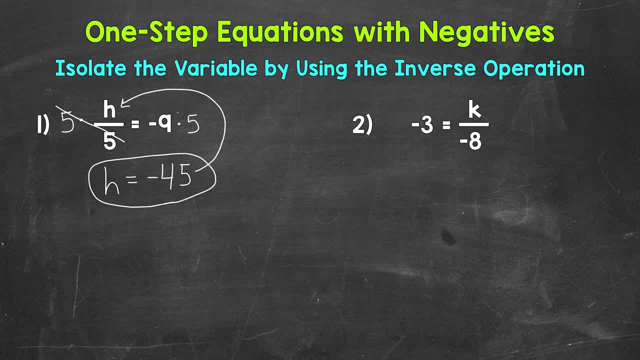 by plugging it into the original equation. So let's plug negative 45 in for h. So we have: negative 45 divided by 5 equals negative 9.. We have a negative divided by a positive, Negative 45 divided by a positive 5.. 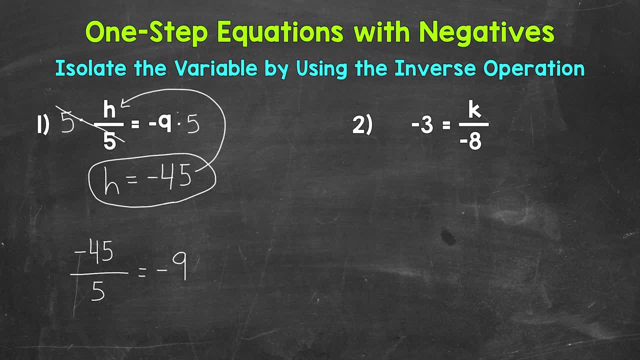 A negative divided by a positive equals a negative Negative 45 divided by 5 does equal negative 9. so we have the correct solution: h equals negative 45.. Let's move on to number 2, where we have negative. 3 equals k divided by negative 8.. We need to isolate that variable of k, Since k is being divided by negative. 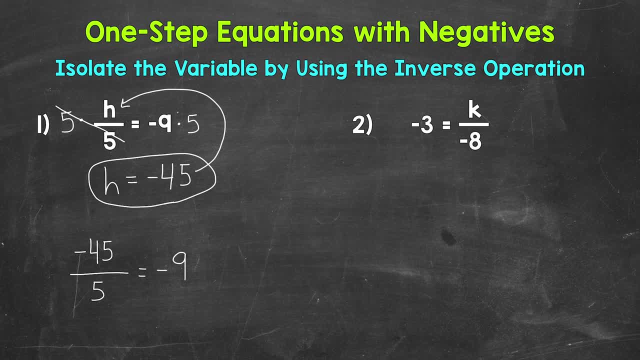 8. we need to undo that division by using the inverse operation. The inverse of division is multiplication. so let's multiply the right side by negative 8.. Whatever we do to one side, we must do to the other. so let's multiply the left side. 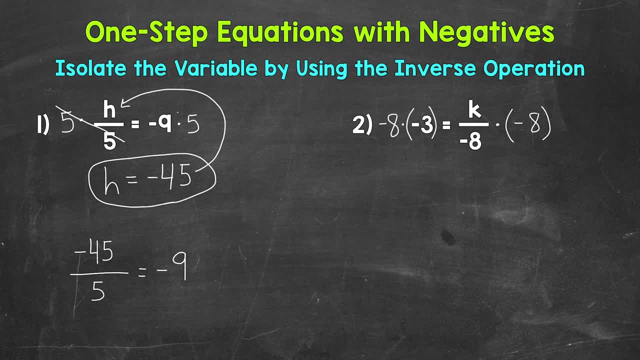 布 we have. That means we have a negative on the other side of the equation. so we Komment view schw vy by negative 8 voters. now, as for the right side of the equation, we are dividing by negative 8 and multiplying by negative 8 so that equals negative 8.. So these negative 8s cancel each other out. They equal 1.. We have negative 8 divided by a negative is a positive, so that gives us positive 1. So we have 1k, which is just k. 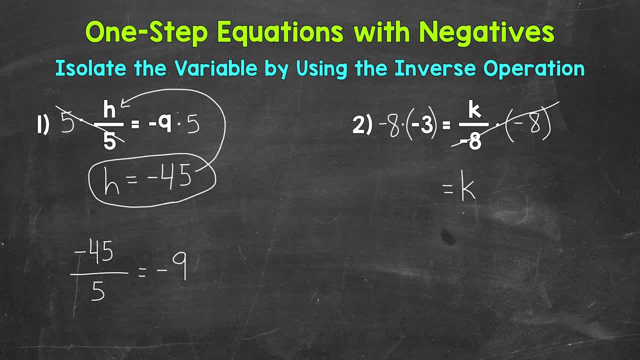 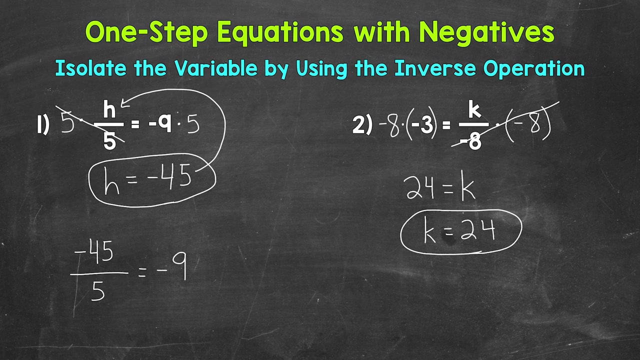 equals. and then on the left side of the equation we have negative 8 times negative, 3 a negative times a negative equals a positive. so this gives us a positive 24. K equals 24, and we can rewrite this with the variable coming first: K equals 24. that's our solution. let's check that solution by plugging it. 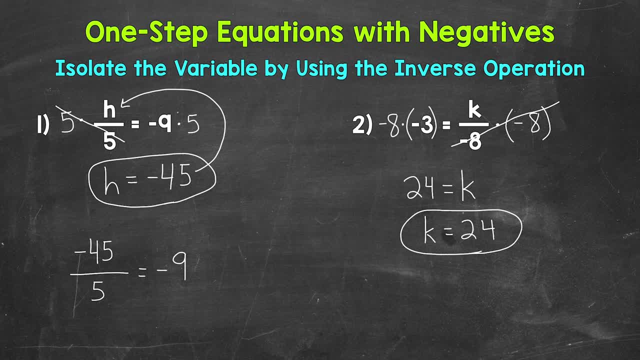 into the original equation. so let's plug in 24 for K. so we have: negative 3 equals 24 divided by negative 8. we have a positive divided by a negative, that's going to equal a negative 24 divided by negative 8 does equal negative 3, so we 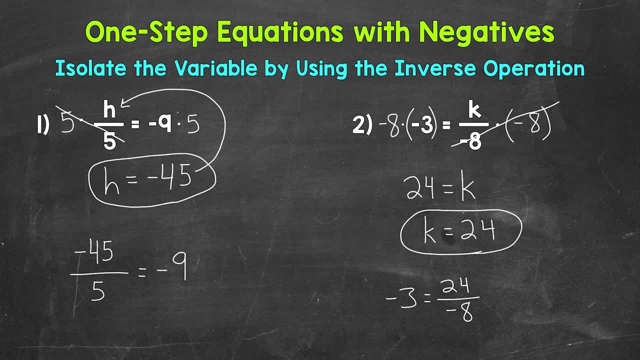 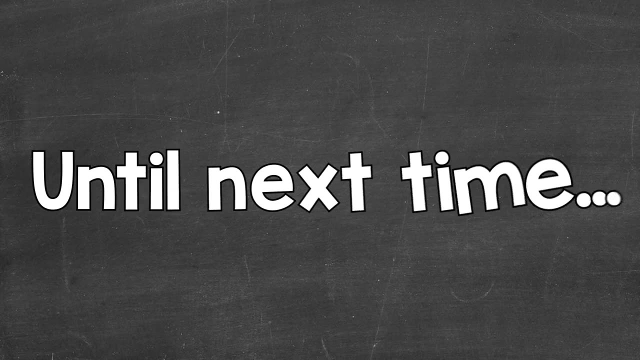 have the correct solution: K equals 24. so there you have it. there's how you solve one step multiplication and division equations with negatives. I hope that helped. thanks so much for watching. until next time, peace.